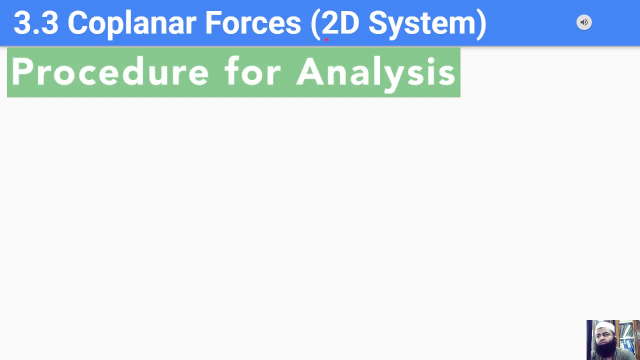 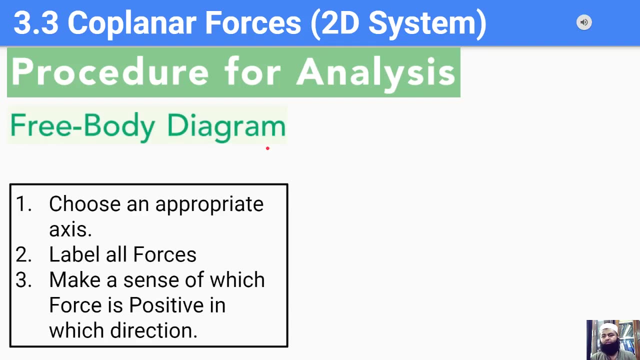 we only consider system of forces, where all the forces are in a plane. Okay, so first, what is the first step? First of all, we draw the free body diagram of whatever the object we are trying to analyze. Okay, like we saw before, what are the steps of drawing a free body diagram? We draw the. 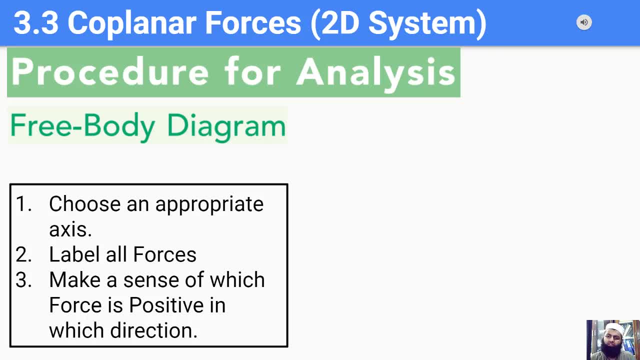 line and then we draw the known and the unknown forces And the next step we want to do is we would choose an appropriate axis. Okay, because now we want to use the Cartesian vector forms. It is very important that we are able to choose some suitable axes for our system And, like before in the free 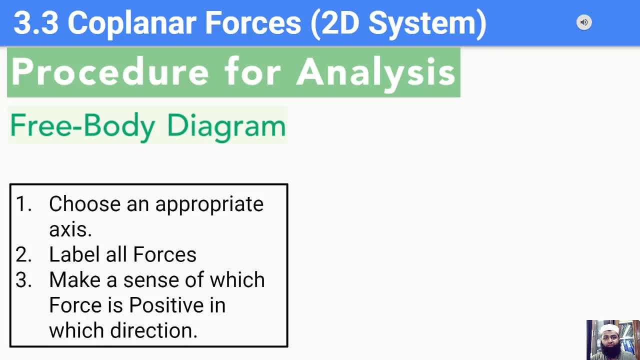 body diagram. we label all the forces And then we choose a positive direction for all of our forces. Okay, so we have to make some kind of a guess for the forces that what these forces are going to be in which direction. Okay, either it is going to be in the positive x direction or the. 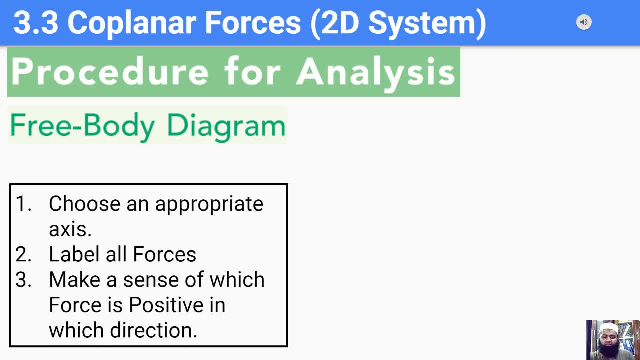 negative x direction, And later we will see that this guess does not really matter for our analysis at the end, But we have to assume some direction in the beginning. Okay, so the next step is that we solve for the two equations of equilibrium. For a two-dimensional system, the only two equations of equilibrium are sum of all the forces of x. 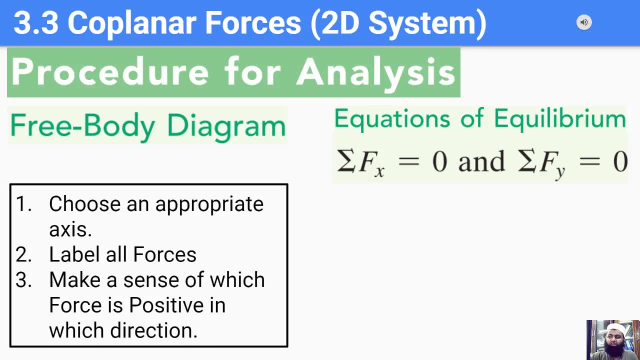 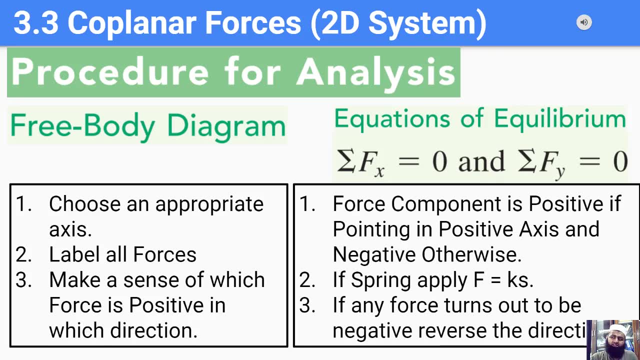 In x are equal to 0 and sum of all the forces in y equals to 0, as shown here. Okay and so, at the end of the day, this, these two equations would be. we would be able to solve these two equations like two simultaneous equations and we would have some unknown forces. Okay, so, once we solve for the 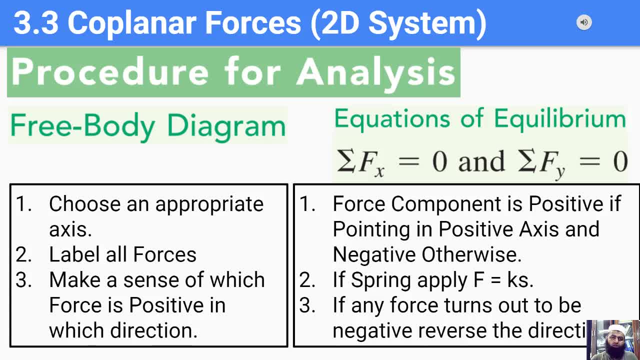 forces, then we can say that we are going to be able to solve for the two equations of equilibrium. So we can say that if the force component comes out to be positive, that means that our initial guess was correct and the force is actually in the direction that we assumed it to be. But if the 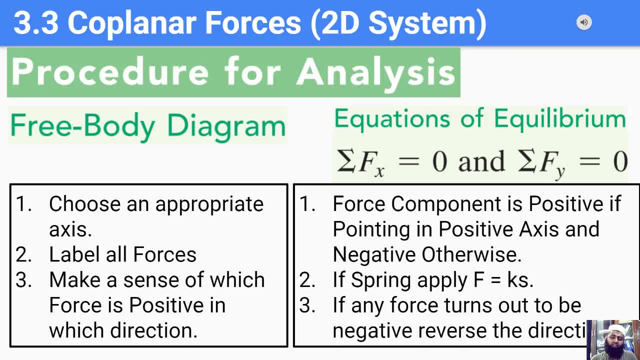 force magnitude comes out to be negative, that just implies that our initial guess was not correct and the actual force is in the opposite direction. Okay, and, like we discussed before, anytime we have a spring in our system, we would just do assume that spring is in the opposite direction. Okay, and 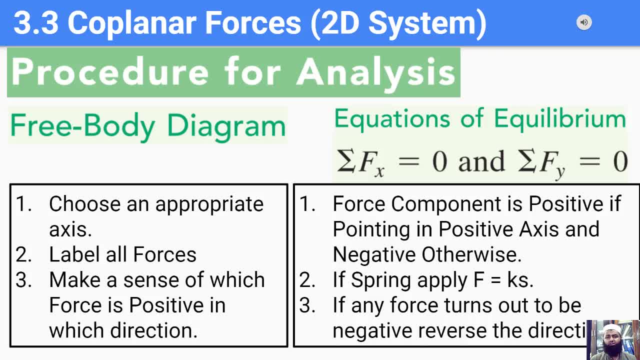 if we assume that spring to be, that it obeys the Hooke's law, which means that force on the spring is equal to the spring constant times, the extension, Okay, as given in the formula here. Okay, as we discussed before, any force that turns out to be negative, we reverse the direction that we 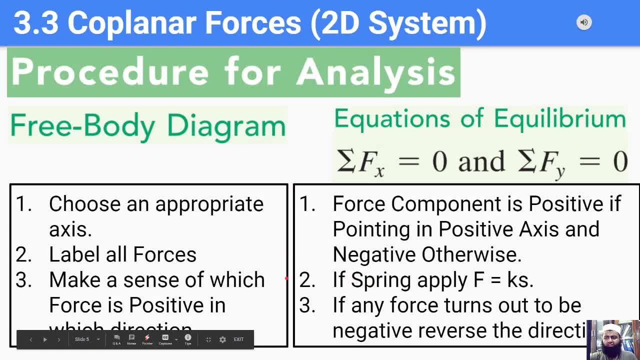 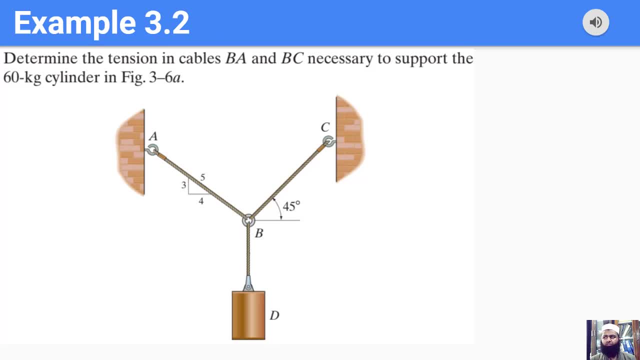 initially assumed. Okay, so this is the procedure of analysis. we would apply this procedure on a few examples To get a clear picture of what we are talking about. Okay, so we here. we have a very, very simple example. It is from the book that determine the tension in cables BA and BC necessary to support 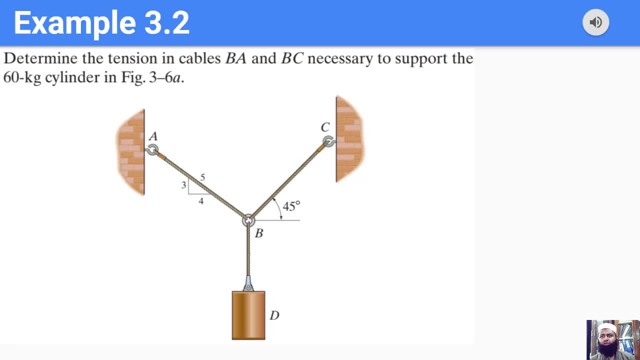 a 60 kilogram cylinder in figure 3.6a. The figure is given below, and now what we have here is that we have a load which is 60 kilograms and there are two strings. One of the string is at an angle of 45 degrees, the other one is at the given through this similar triangle, as we discussed before, and now we want to solve for these three forces. 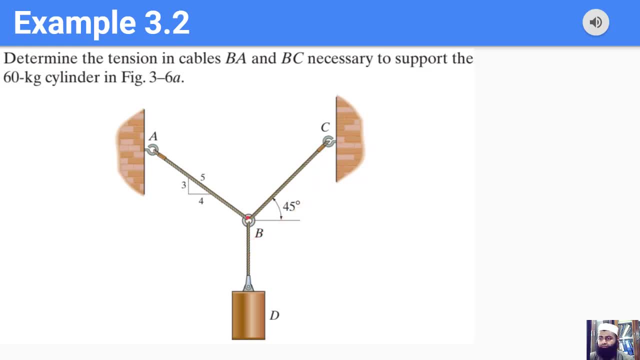 So what was our first step? So the first step, as we discussed earlier, was to draw the free body diagram. Okay, So, let's see, Okay, So let's see, we want to draw the free body diagram of this ring here. Okay, because these all the three forces are acting on this ring, the most appropriate free body diagram would be for this ring. 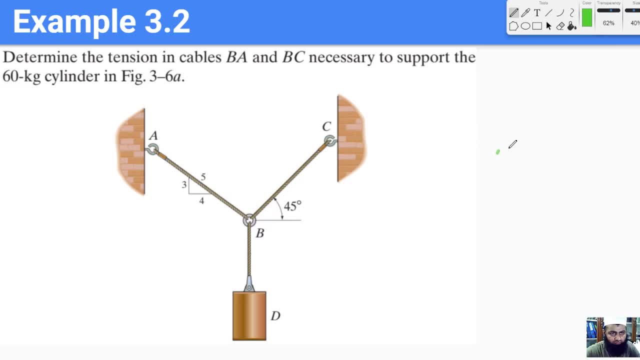 Okay, so let's start. So first of all we draw the outline of the ring. So here we have the outline of the ring, and then we draw all the forces acting on the ring. Okay, Okay And so. So let me draw the forces with something like a red, and the first force is the force due to this mass here, and so this is going to be 600 newton. 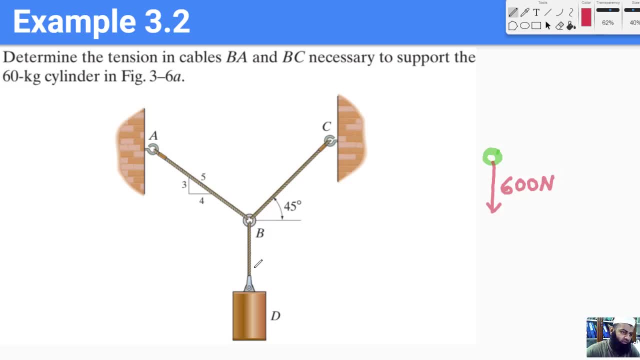 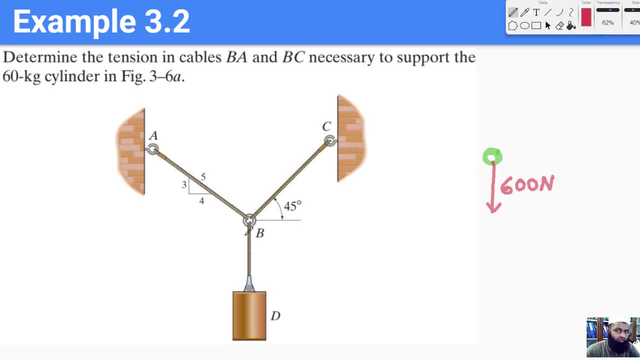 And then same tension applies here. but we can keep that step and we can just say that the force here is the same as the weight here. Okay, The second force is going to be in this direction, and let's just call it FC, because this is acting towards this point C. 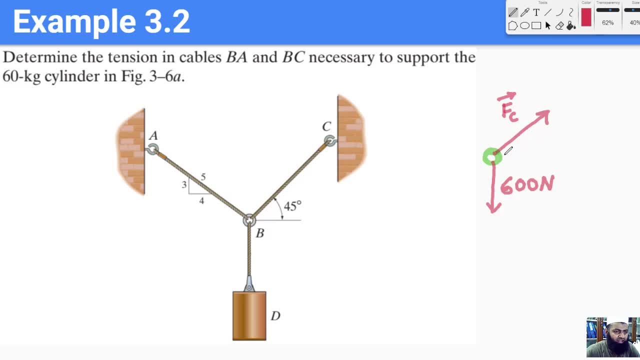 Again, the name is pretty arbitrary. You can choose two names. I would choose correct, whatever name you like, but this is one naming system that I like. the second force is in the other direction, and again we draw the same similar triangle here. so this is 5, 3 and 4. okay, so now I have drawn the free body diagram. okay, so. 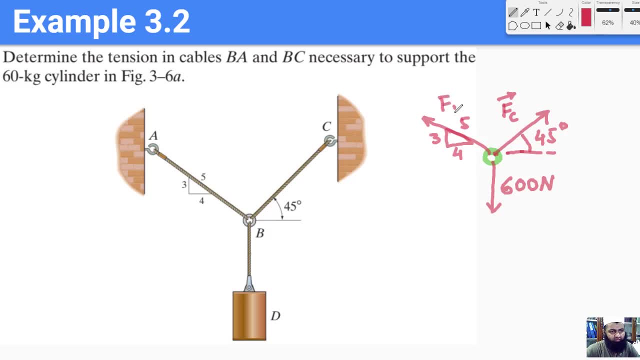 I have to label this force also, so I call this F B. okay, so these are all the three forces acting on this way. the next step, as we saw earlier, is to let me- okay, and now I want to draw an axis. okay, the most obvious choice for an axis is: 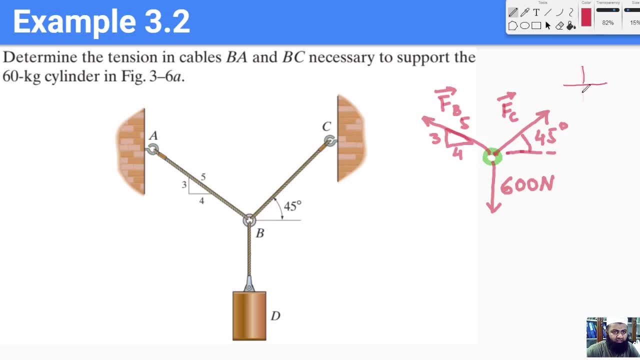 to simply draw the axis like this. so this is my x-axis and this is my y-axis, okay, and I am assuming that my positive axing is in this direction. the positive Y is in this direction. again, this is a pretty arbitrary choice. I can choose any type. 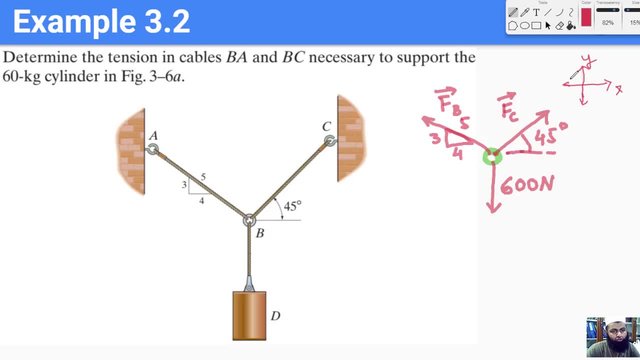 of axis that I like, but of course, this is the most common choice that most people make and this is the most common choice most of us making. okay, so the next step is to apply the equations of equilibrium. so the first equation is that sum of all the forces in X equals to zero. so how many forces do we have in? 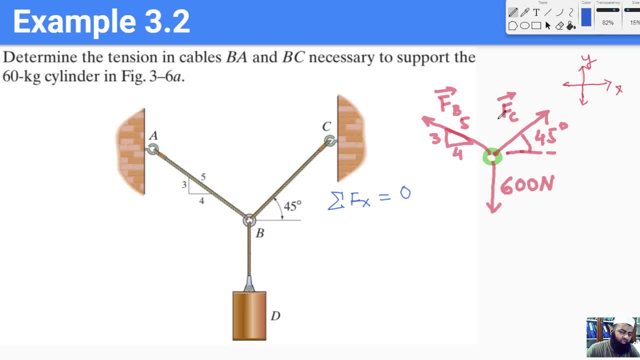 X. we have a X component of the force FC and we have an X component of the force FB. so FC times cos of 45. this is the X component of the force FC. again, because I am NOT putting an arrow here, this means that this is a magnitude okay and 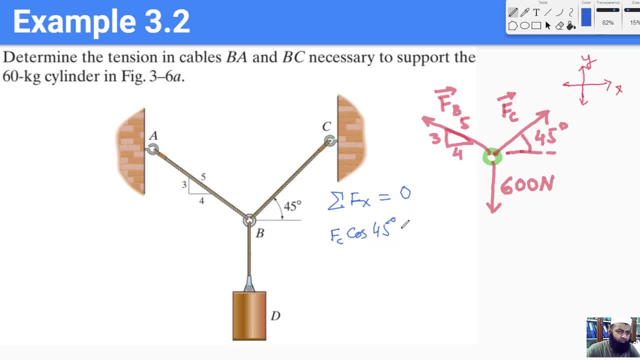 the second force is is going to be in the negative direction, because this force is the X component of this forces in the negative direction. so, and because this is going to be a cos of theta, and which is equal to 4 over 5, and this equals to 0. so this is our first equation. 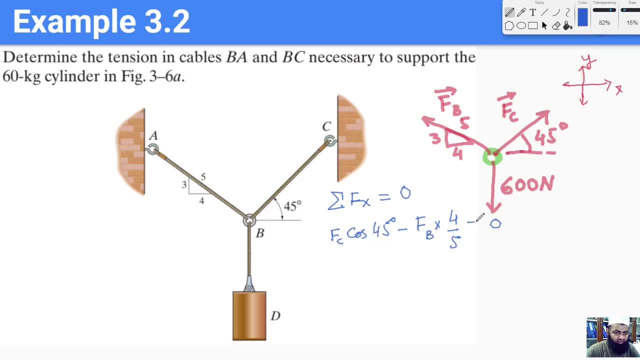 let me just correct my okay. so the second equation is the equation in the Y axis. and the Y axis we have three forces: the for the Y component of FC, the Y component of FP, and this force is also in the Y direction. so now for we say FC. 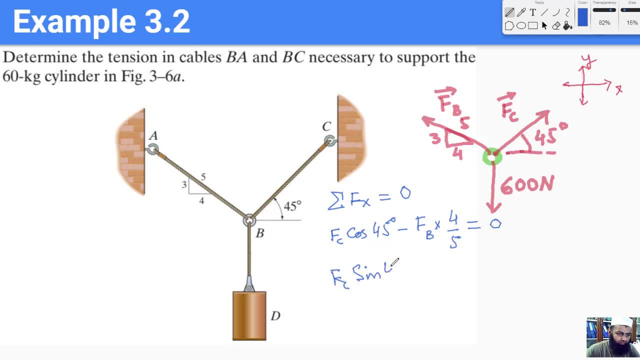 sine of 45 degrees alten minus O times 반, or I get theBy' BTS sine of 43. Deus對啊, diretty proced shigh for hetera plus fc, %EF, PM O N plus Y dA, plus FB times, 3 over 5, and so now this is in the minus direction, so I would say minus 600. 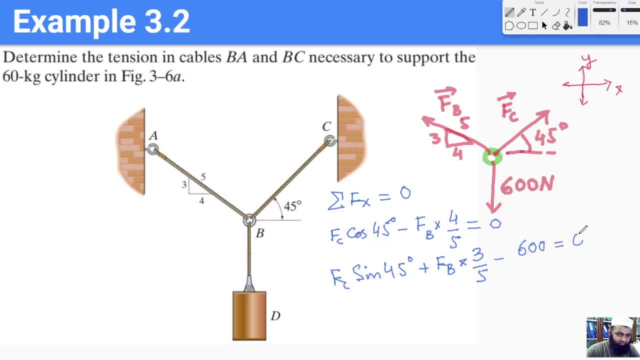 equals 0.. So here we have these two simultaneous equations. So these are two simultaneous equations and there are two unknowns. So two simultaneous equations with two unknowns. we already know how to solve them. You might have learned how to. 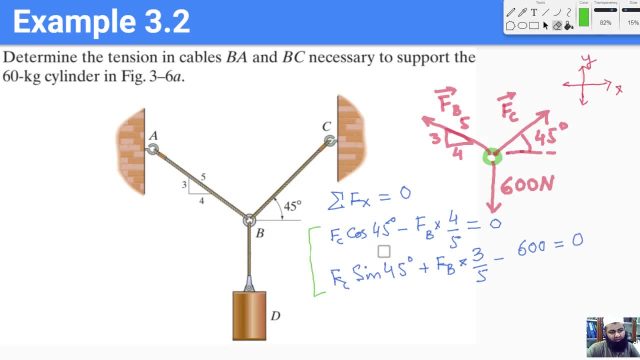 solve them in your maybe 7th or 8th grade. So I hope you can find FC and FB given time So you can find these equations. One of the easiest method is because sine of 45 degrees is equal to the cos of 45 degrees, So we can just subtract the two equations and then 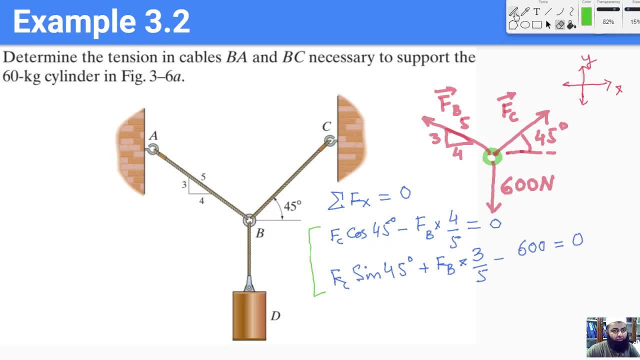 we just get an equation for FB. Once we have solved for FB, then we can plug it in one of these equations to find the value of FC. So I hope this is pretty clear. Nothing very fancy here. So now I think all the steps should have been very, very clear. First of all, we draw the 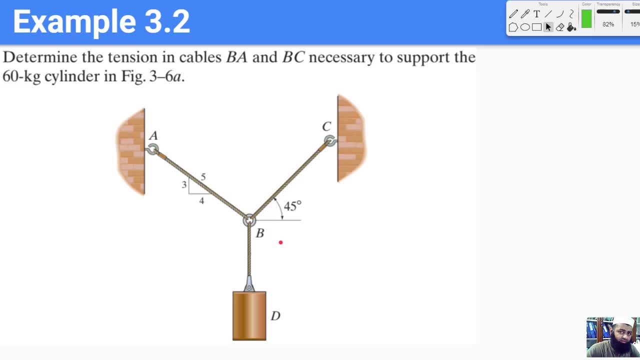 free body diagram, then we choose an axis, and once we have done both of those things, then we apply the equations of equilibrium. So here is the two free body diagrams. Again, like I discussed before that, we have avoided making this free body diagram because we know that for a block in 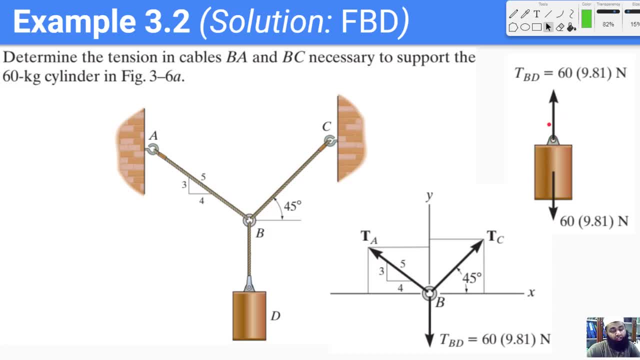 equilibrium which has only two forces, are going to be equal, which means that the weight of the block is going to be equal to the tension in the strain and that tension is going to be the same tension which comes out to be here. This is an extra step which we would- we can avoid also. 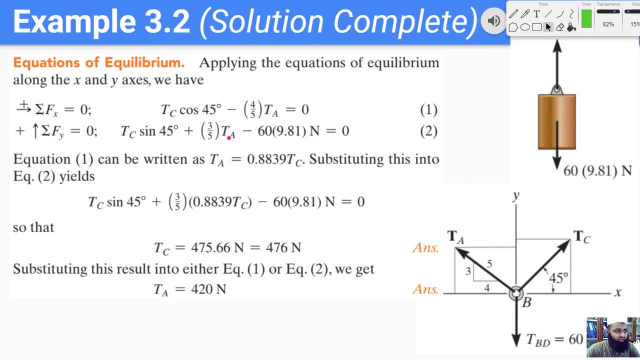 So here is the working. So we get similar equations like this Again in the book. they are using the value of 9.81.. The values are 9.81.. So you know it is not necessarily true. So this is not necessarily true. So here is the working. So we get similar equations like this Again in the book. they are using the value of 9.81.. 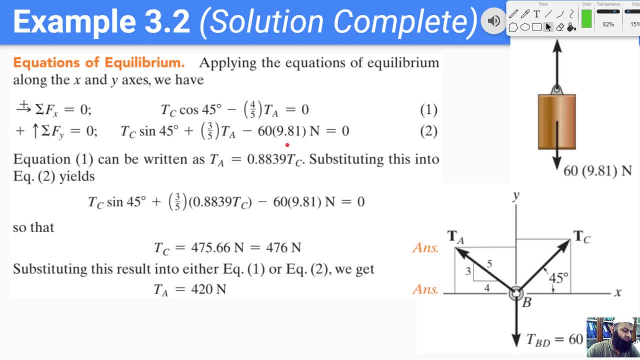 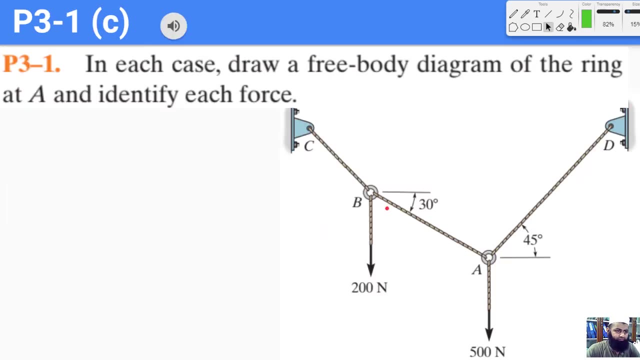 the value of g, but for this course we would use the value to be 10 meter per second square, which means that some of our answers would be a little bit different from what we have in the book. So here is another example. we want to draw the free body diagram of the ring A and identify: 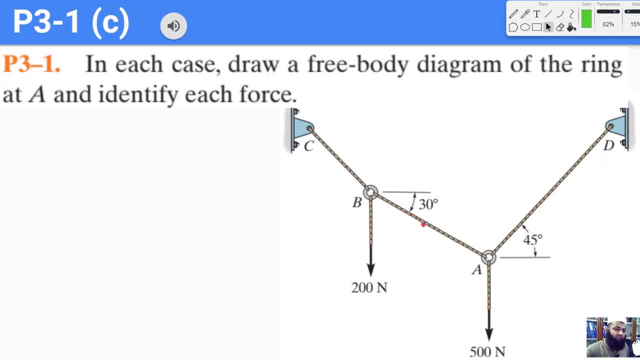 each of the force. Now here, we are not required to solve the free body diagram, because we are just required to draw the free body diagram. So we want to draw the free body diagram of this ring. So let's see how do we do that. 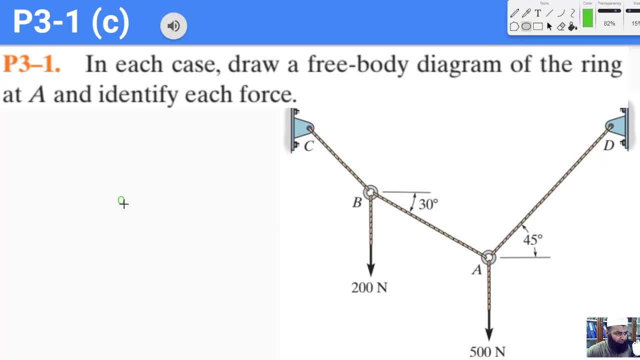 Let me try to draw a ring using the circle. That's much better. So now we have this ring. and how many forces? again, I would like to draw my forces with the red, Okay, and my downward force is the 500 Newton force, which is already given here and then. 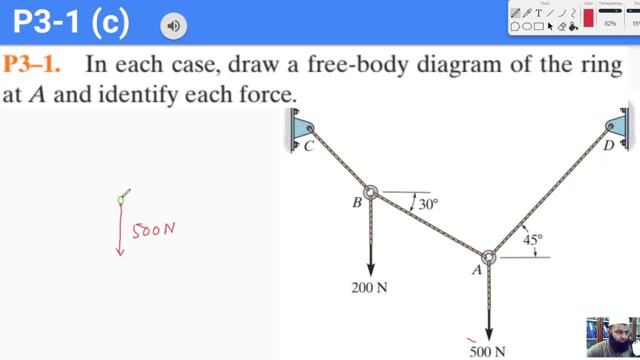 they are going to be two unknown forces. One of the force is going to be in this direction, at an angle of 45 degrees, and this force is- I will call it- Ft, Because it is going towards D. Some people also use the term FdA, which means that this: 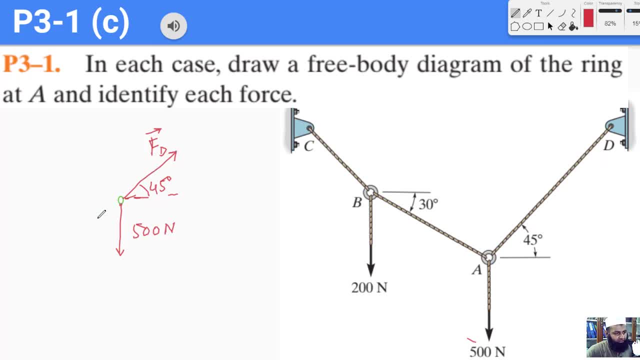 is a force towards D from A, but it's a choice that you can make. This third force is in this direction. Again, my forces- because I am using a stylus- is these are not as straight as they should be, but I hope you understand that this force is a straight line. 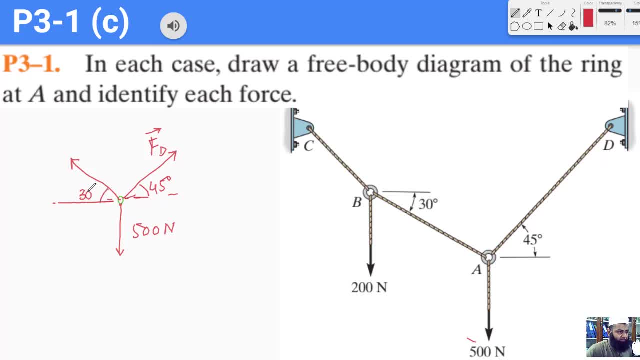 Okay, And this angle is again 30 degrees. Okay, And this angle is again 30 degrees because this angle is going to be equal to this angle And I call this force as Fd. So here I have drawn the free body diagram of this ring A. I have identified all of the 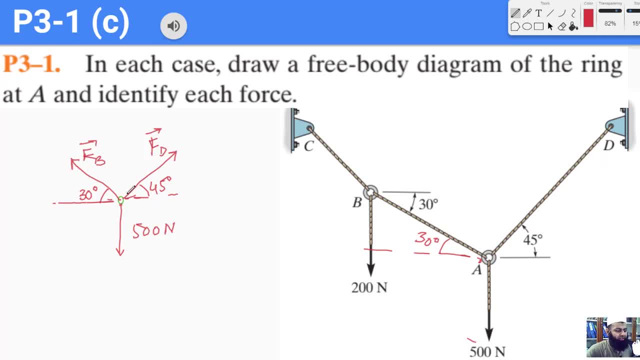 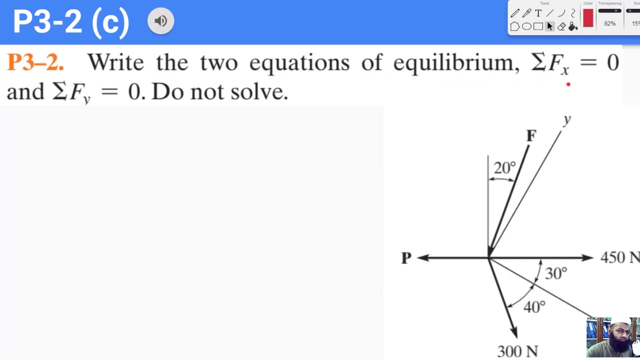 forces. Notice, we do not need to define an axis, just to draw a free body diagram. We need to define an axis to solve using the Cartesian vector form. Okay, Moving on Now, this is write two equations for equilibrium: sum of x. forces in x are equal to 0 and sum. 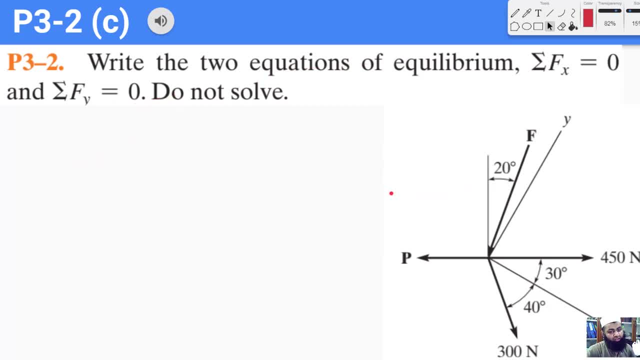 of the forces in y are equal to 0.. Here we are only concerned with writing the equations, Okay, And we are not really concerned with solving them. Okay, Okay, So we have these two axes. The tricky part in this problem is that the two axes are- they are still perpendicular to. 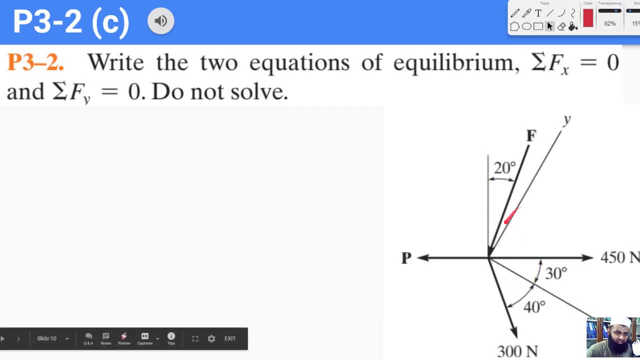 each other. but they are making this funny. they are not the usual vertical axis and horizontal axis, Okay. So let me just clarify a few things so that we are able to solve. Okay, We are. we know that this angle is 90 degrees. 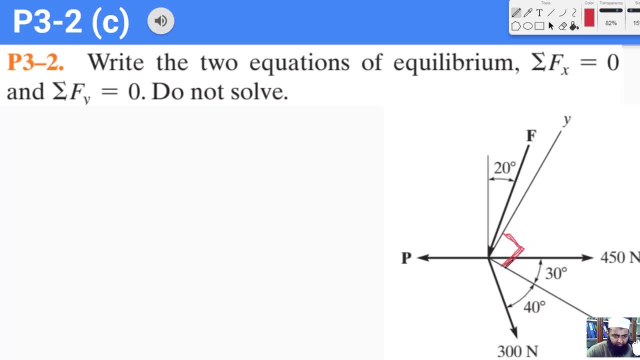 Okay, And I am trying to draw a block here. And secondly, we also know that this angle is equal to 90 degrees. Okay, So this is the only two information, that, and the other angles are already given. So now, first of all, we would write- try to write the equation for: sum of all the forces. 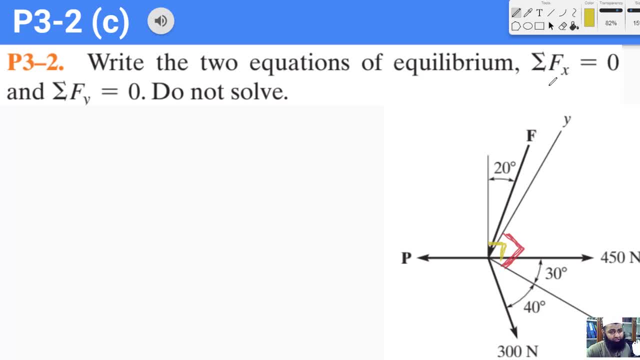 in x are equal to 0.. Okay, So how many forces do we have? We have this force P, we have this force 400 Newton, 300 Newton and this force F. So what is the component of this 400 Newton force in the x direction? 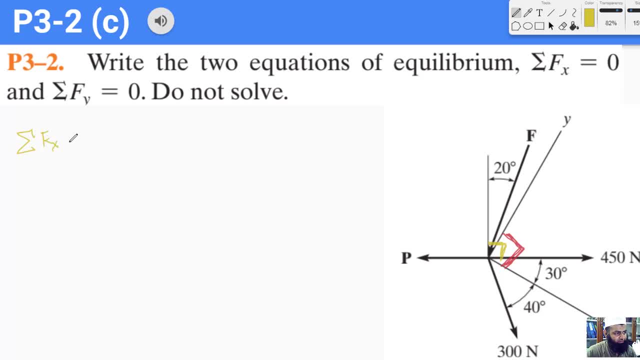 So let us say that sum of all the forces in x equals to: so this is 450 cos of 30 degrees. That is the first equation, First component of our equation. This one is minus 300, actually plus because x component is plus y component of this 300. 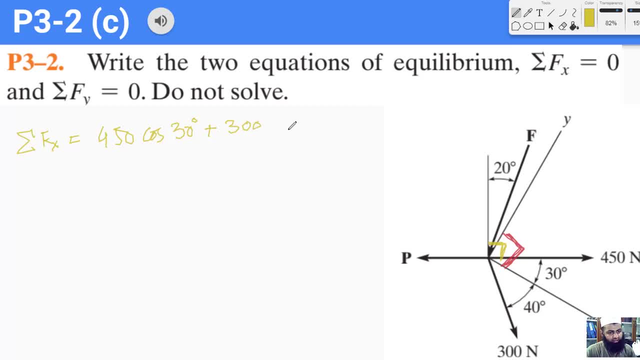 force is negative. Okay, So 300, and then we have cosine of 40 degrees. Okay, So these are the two terms. Then we want to find the x component of this force, P- I can extrapolate the x axis here- And so this angle again is going to be 30 degrees, which means that the x component of 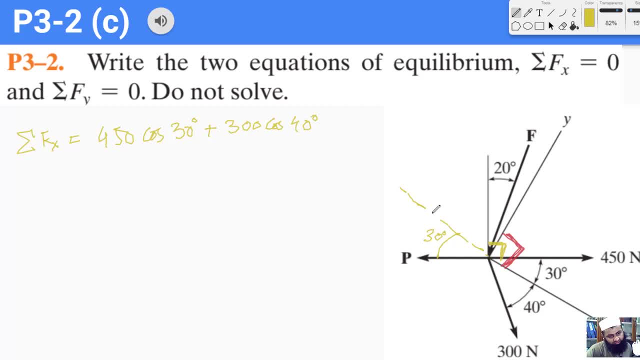 P is going to be negative, It is going to be in the opposite direction. So I say minus P, and then we say cos of 30 degrees. Okay, And so the last equation, the last force, is this force, F, And so this is making an angle. 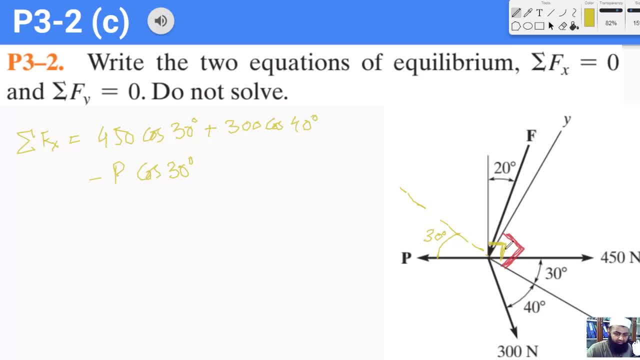 of 20 degrees with this perpendicular, Okay. So now we have to figure out the angle that this means. So this angle is 90 degrees, which means that this angle is 60 degrees, Okay. And because this whole thing is 90 degrees, which means that this angle is 10 degrees. 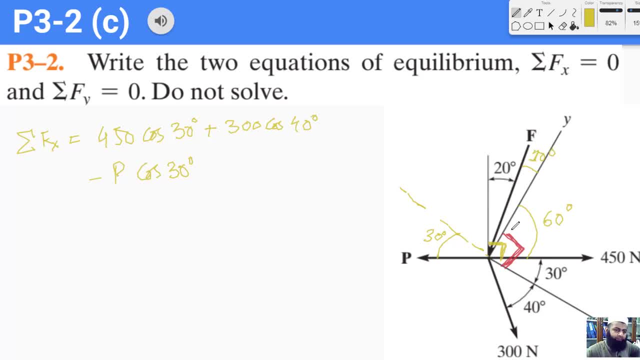 Okay, This is again very, very simple trigonometry. You would have been very, very familiar with this Already. So this means that this force F makes an angle of 10 degrees with the y axis, And it's because it is pointing in this direction, which means it's x component is going to be: 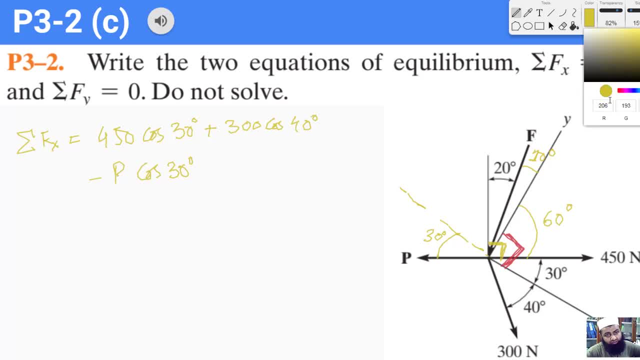 positive. So it's x component. Let me choose a different color. So it's x component is this and it's y component is: is this okay? So it's x component is going to be positive, but it's y component is going to be negative. 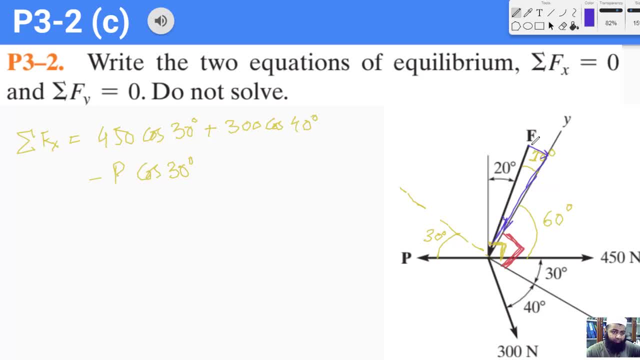 Okay, So now the x component of this force, F, is going to be plus F, And now we have sine of 10 degrees again, because here we see that we are trying to measure this length. Okay, So this is the first equation. 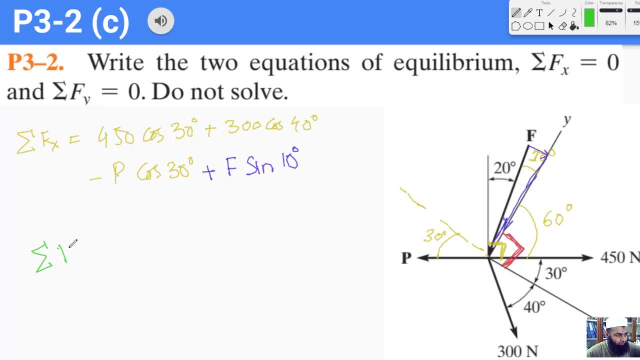 Let's go back and write the second one, And sum of all the forces in y is equal to 10 degrees. Okay, So this is the first equation This is equal to. so the first force is going to be for 50, this, this is just positive. 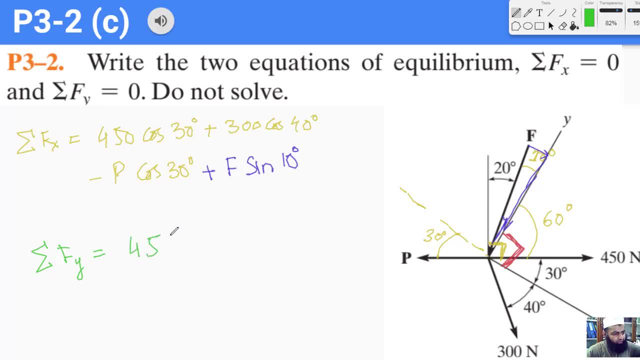 in y direction. So that is going to be four: 50- sign of 30 degrees. This force is going to be in the negative direction, y direction. So now this is going to be minus 300- sign of 40 degrees, And this is also in the negative direction. 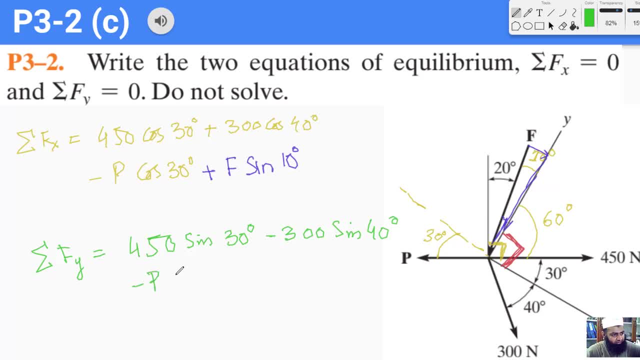 Which means that is minus P sine of 30 degrees. And the last force: again, this also has a negative component, which means minus F times cos of 10 degrees. Okay, So these are the two equations of motion. Okay, So, these are the two equations of motion. 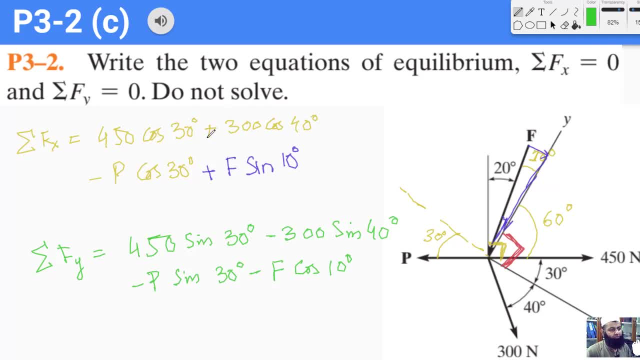 Okay, So this already states that we do not want to solve these equations. we just want to write these equations, And now, once we have these equations, you can already see that it is not actually very, very difficult to solve them also, So they become an equation when I say that this is equal to 0.